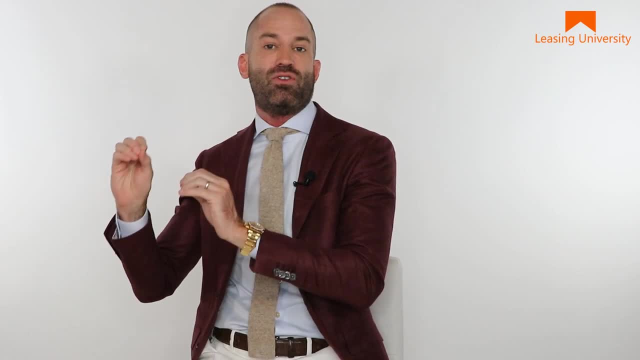 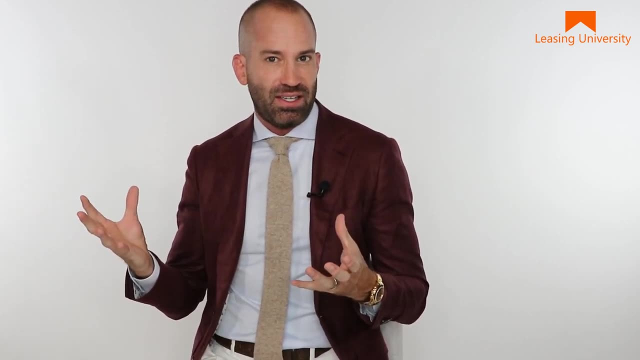 There's a lot of outdated information and there's a lot of downright misinformation out there. The stuff that worked in the past to close leases, well, it's the wrong stuff today. It just doesn't work. Today's renter has to close a lease. It's the wrong stuff. Today's renter has to close a. 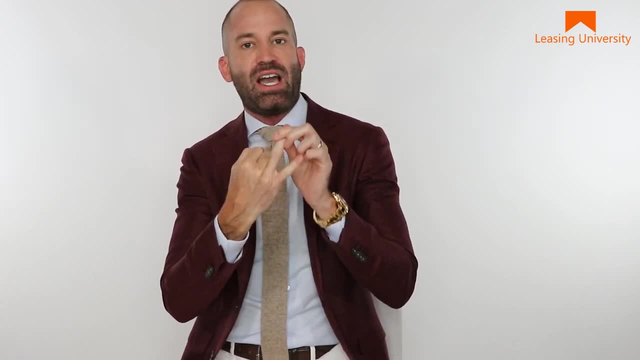 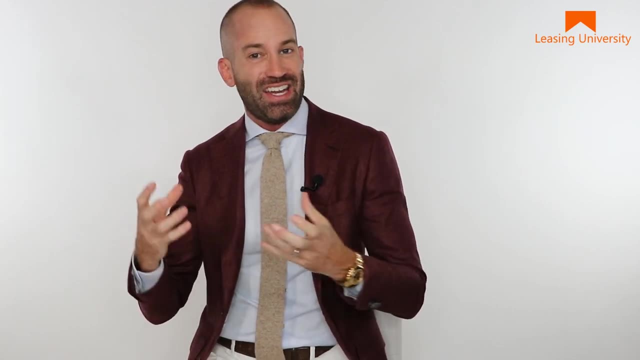 lease. Today's renter has more access to information than ever before and they've got more choices. So that old school way of trying to sell them on the apartment in many cases not only is it wrong, but it actually turns your prospects off and turns them away. 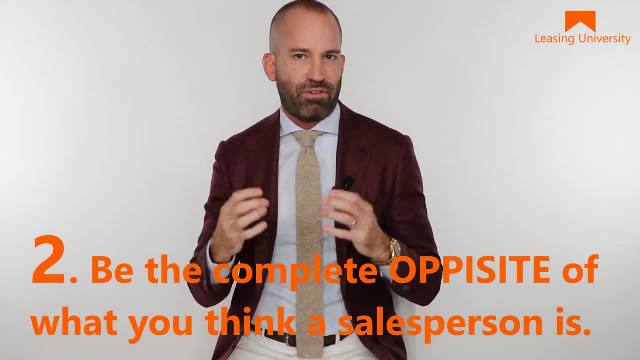 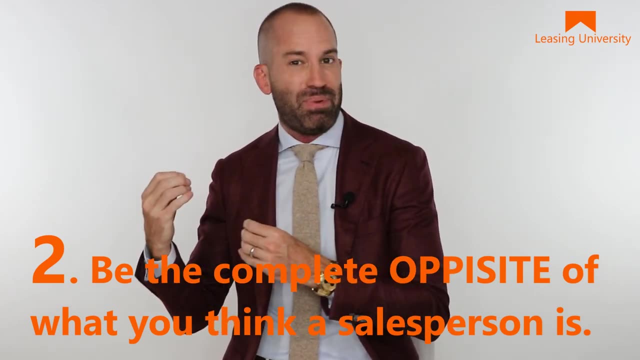 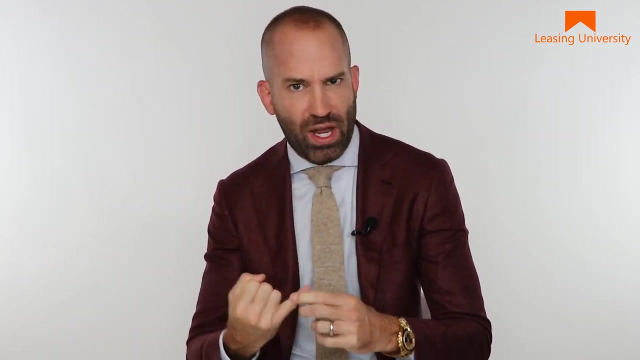 Number two: selling is so important for property management professionals We've got to sell our prospects on living at our community. I want you to be the opposite of what you think a sales person is right. That kind of high pressure, hey, if you don't rent the apartment right now? 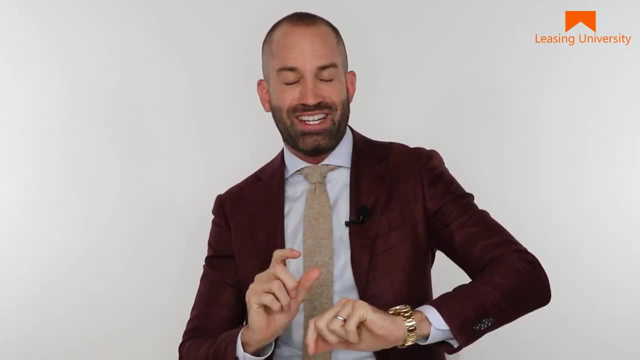 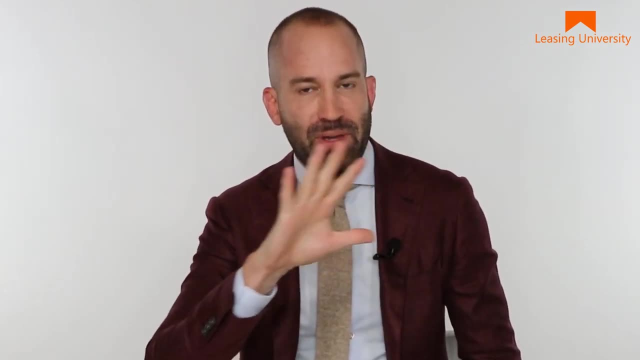 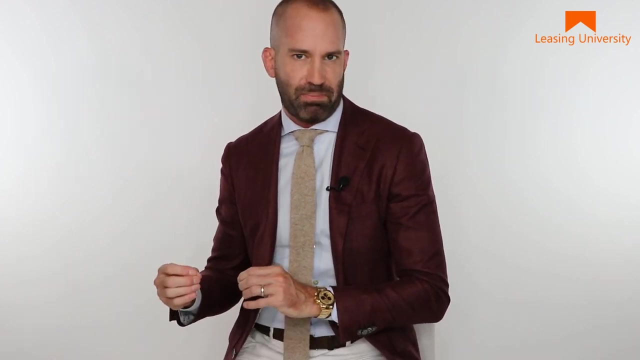 it's going away and we've got a special. It ends in three minutes. How you think of a salesperson, that kind of traditional character from the movies? yeah, be the opposite of that. In today's world, what makes an effective property manager is somebody who can read people. 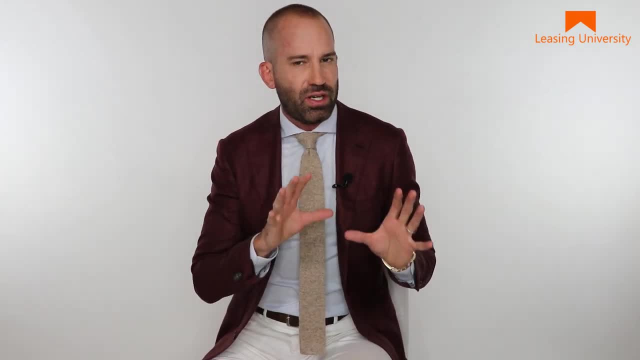 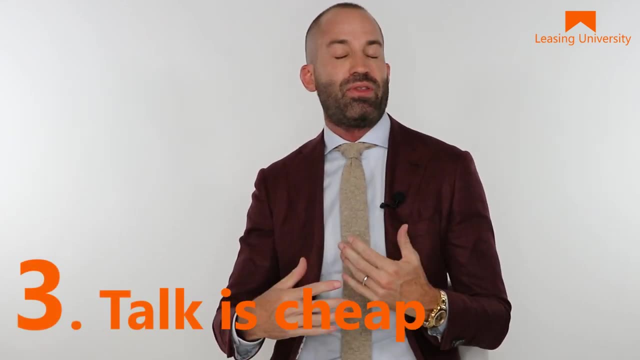 somebody that's able to follow a process, who can engage their prospects in a conversation using a systematic approach. Number three: talk is cheap. A lot of people think that having that kind of gift of gab, being able to shoot the breeze and have all kinds of small talk with our prospects- 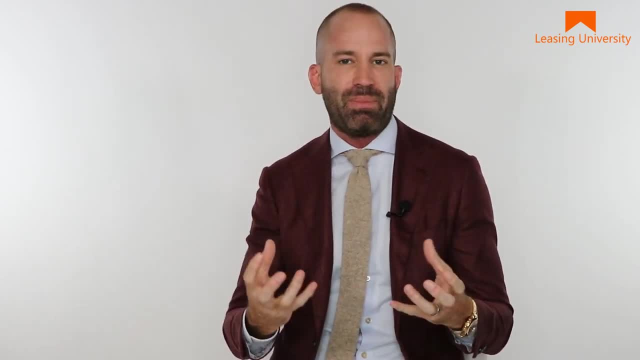 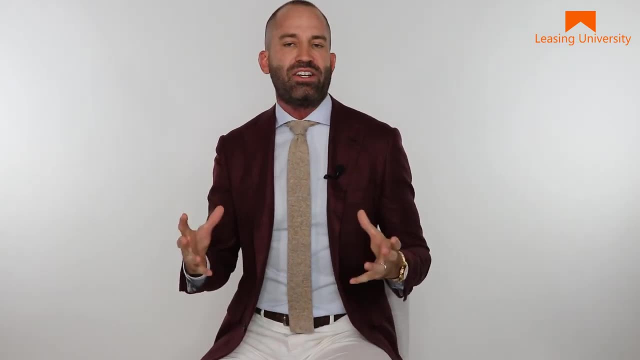 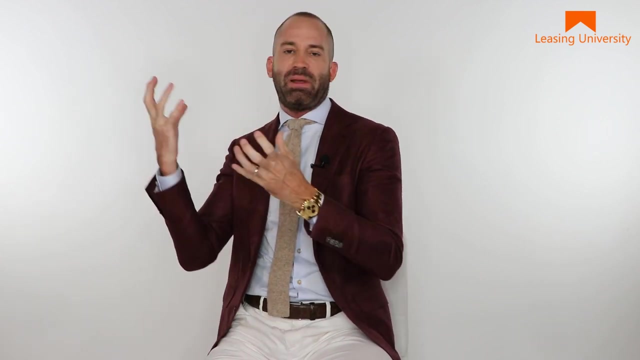 is so key to building a relationship and leasing them an apartment. Well, it's not. The reality is your prospects don't want to hear you talk. They don't care about you. They don't care about the list of amenities that you have. They don't really care about the specials that 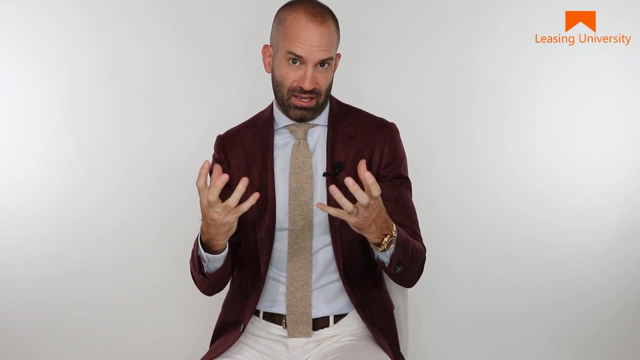 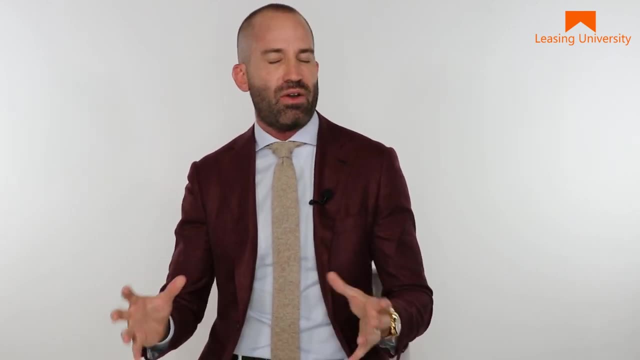 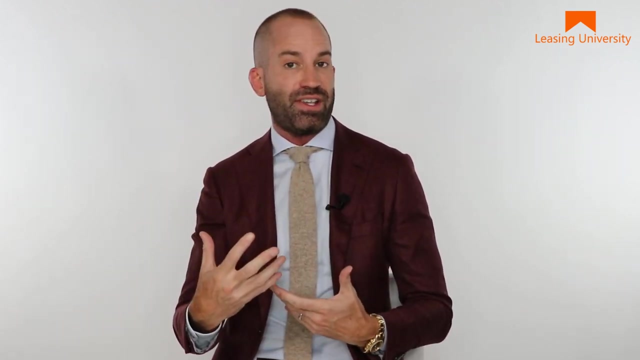 are going on and all the things that you think might be enticing to them. What they care about is solving the challenges that they're dealing with right now, and they're going through the process of moving, which is a very stressful life event. They're looking to connect with somebody that's going to listen a lot more than 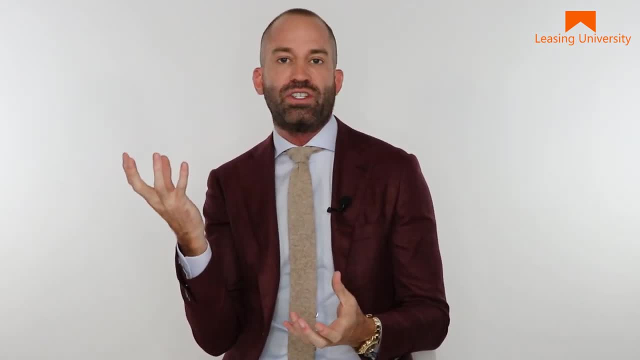 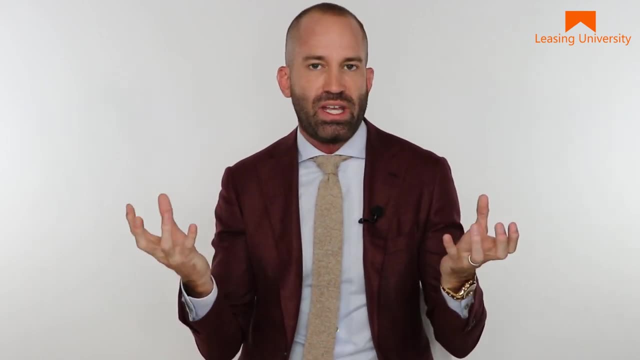 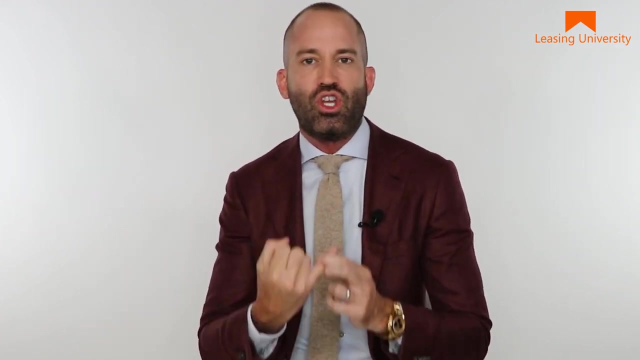 speak and somebody that's truly going to understand what their current situation is and how they can improve it, how they can get that ideal scene. They really don't care about all the things that you have to say until you understand them. Listen, people don't care how much you know. 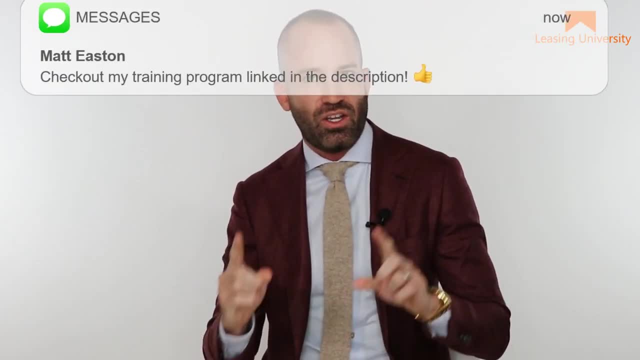 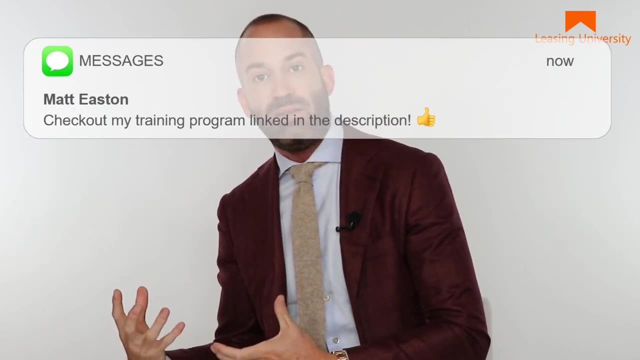 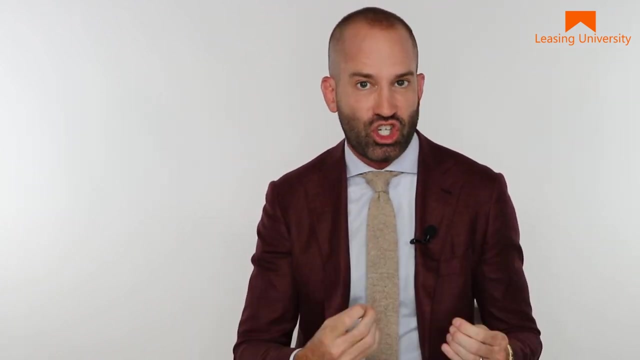 until they know how much you care. And going back to what you've been taught is wrong. we've been trained in this industry to automatically, as soon as we get a tiny bit of information, start talking, start pitching, start selling. Well, talk is cheap. You need to. 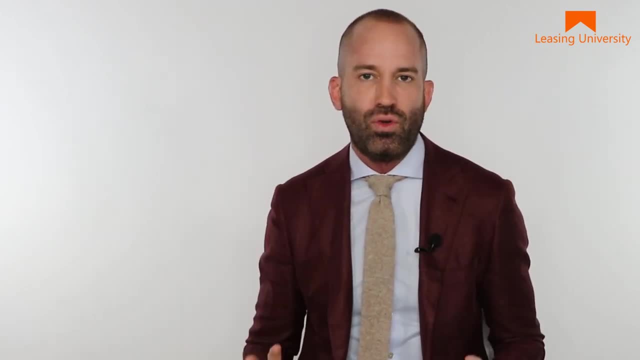 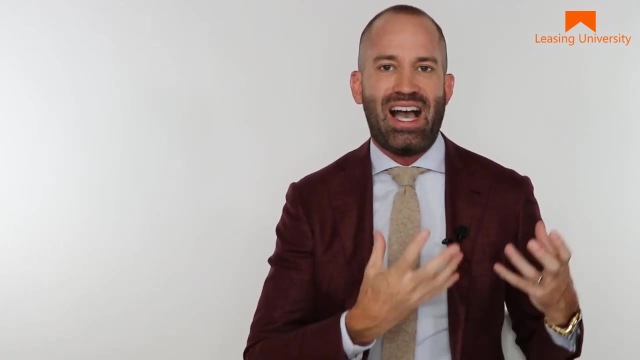 ask the right questions and you've got to dig in. You've got to ask the right questions and you've got to dig in And truly understand not only your prospect's situation but what they're going through and the ideal living situation they're trying to get to. Number four: have a system As a relatively 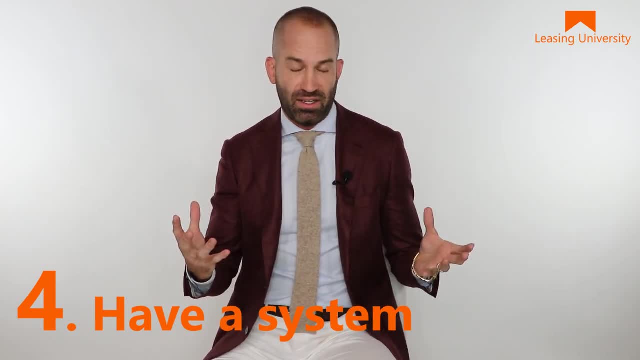 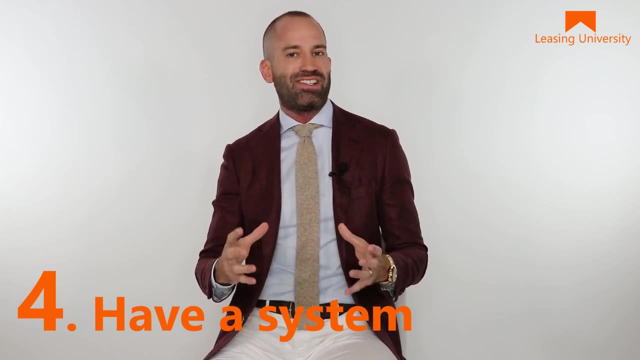 new property manager and even as kind of an OG that's been in the industry for 25 years. the best thing that you can do for yourself is to have a proven system, a process that you trust, a system that you follow. You follow that system and you can do that for yourself. 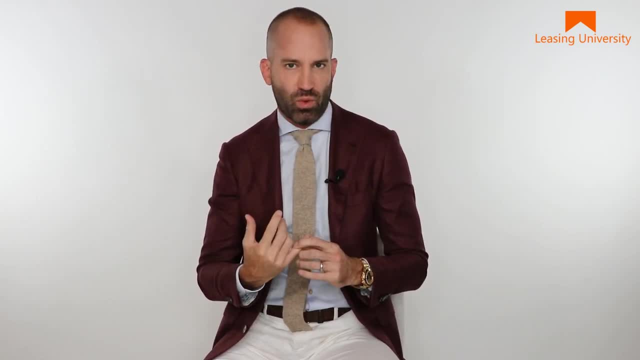 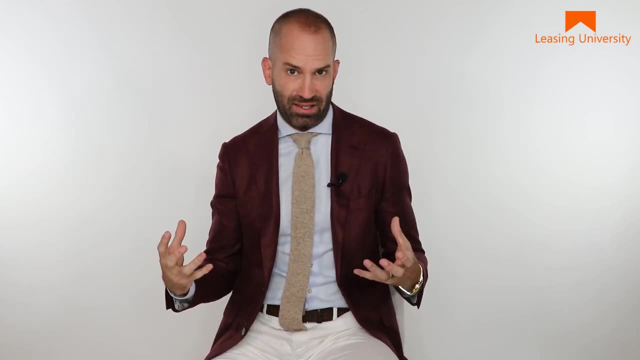 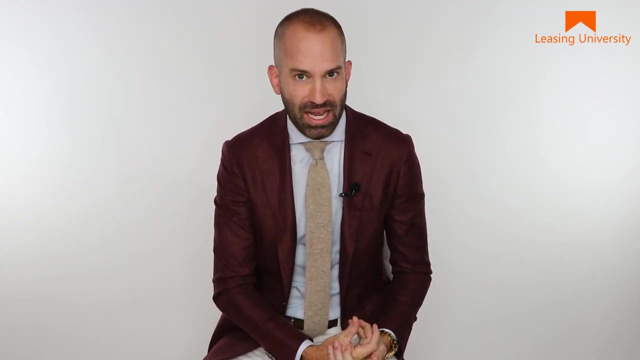 process. so you know exactly where each and every one of your deals is, in what stage of the process that they're in. a lot of times people try to wing it. remember this is a stressful life event. it's also the most expensive decision that your prospects are going to make. just winging it is not going to get you. 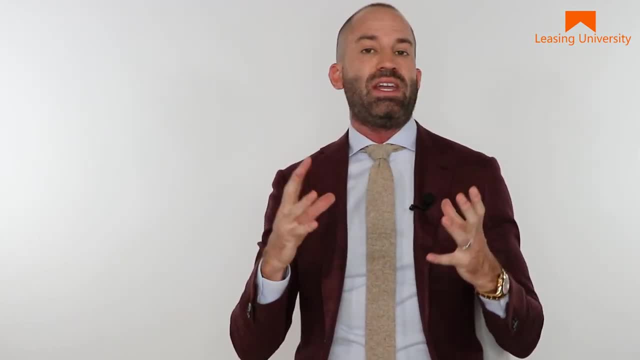 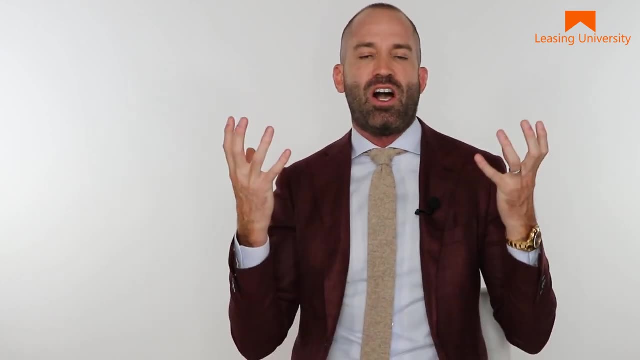 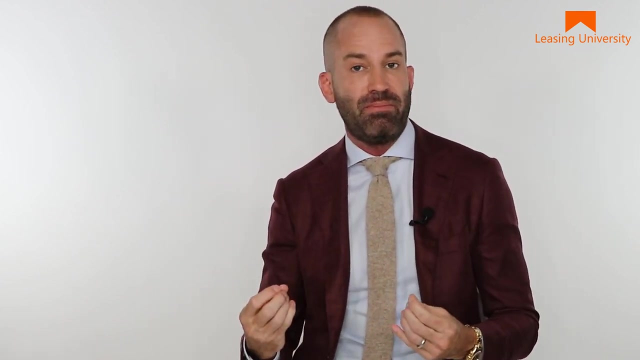 there. you need to have a system and, just to add to that, you want to make sure that you have a system that's been proven to work in today's world, as we said before, the entire apartment industry has changed, and it's changed in the last couple years, so make sure that you have a system that's relevant for. 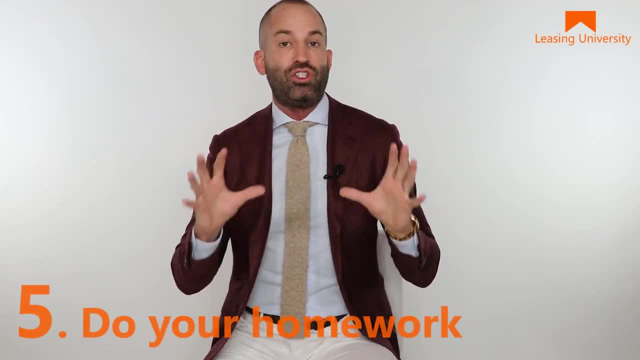 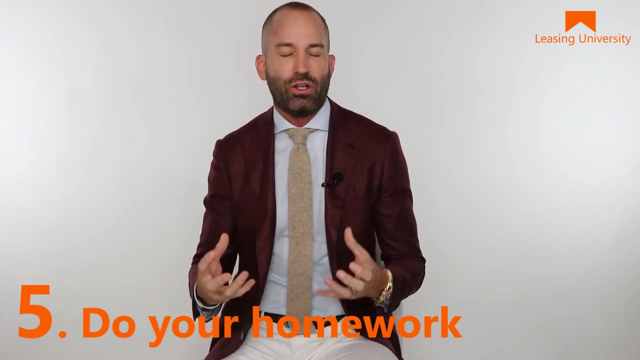 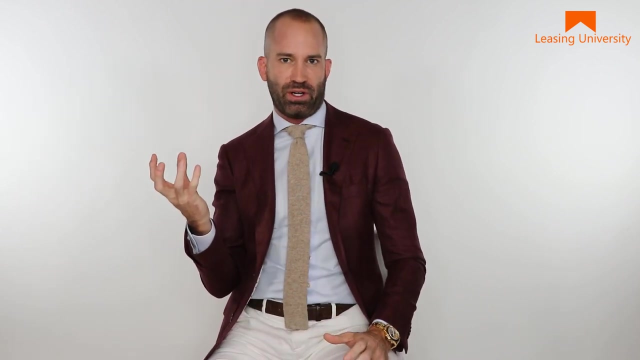 today, relevant for right now. number five: do your homework. show your prospects through personalization, that you truly have taken the time to learn about them, that you understand their current situation. you know what's most important to them and why that's important to them. you know what they want to see. 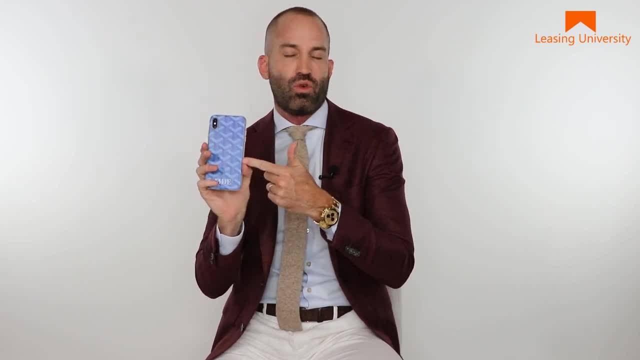 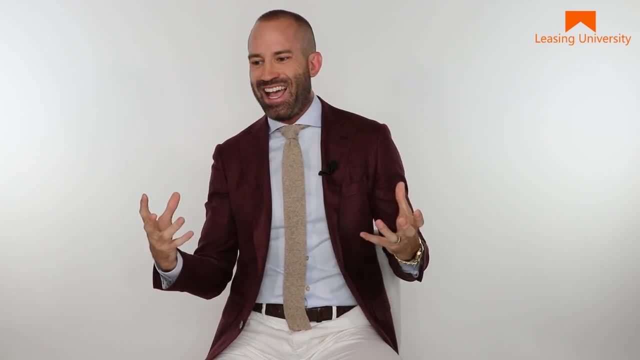 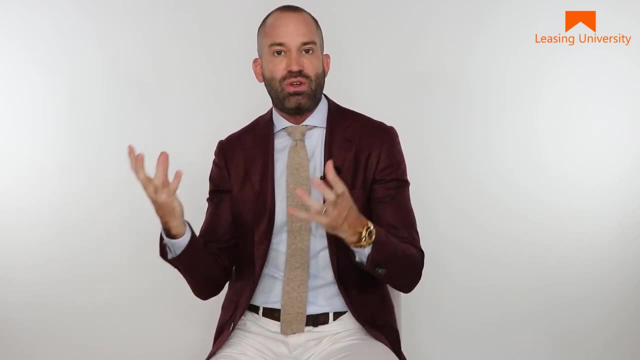 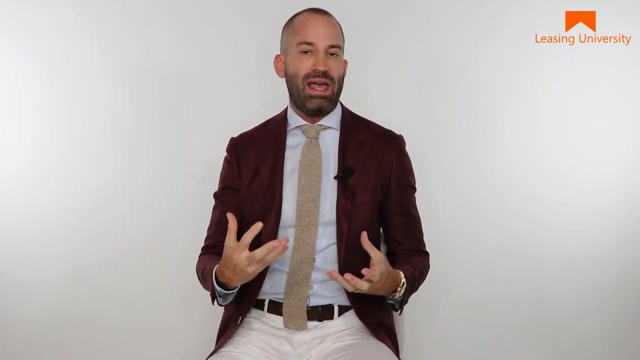 your homework now, that's not. I'm not asking you to sit down for 30 minutes and try and like be a private detective and learn about somebody you've never met before. you can easily do your homework right from that first phone call, even from a chat interaction, from a web form, if you know what questions to ask in the. 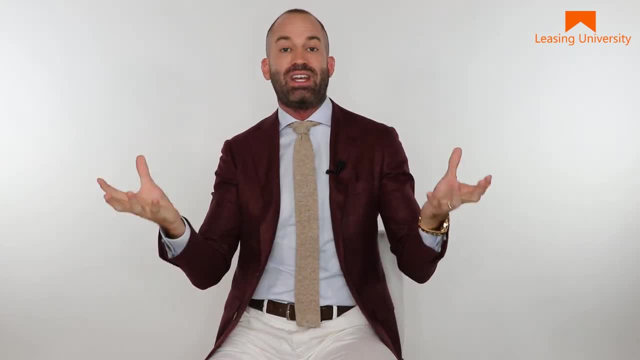 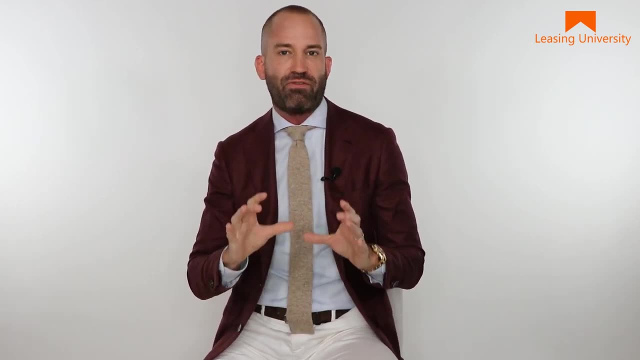 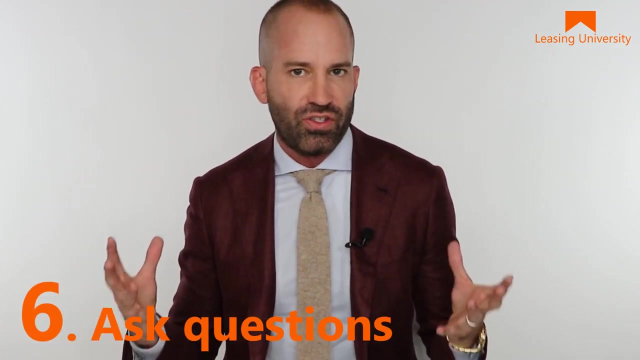 right order to ask them. you can do your homework so that every one of your tours, every one of your engagements with a prospect is personalized just for them. that's gonna set you apart from the competition number six. ask questions, and of course, not all questions are created equal. make sure that you have a system. 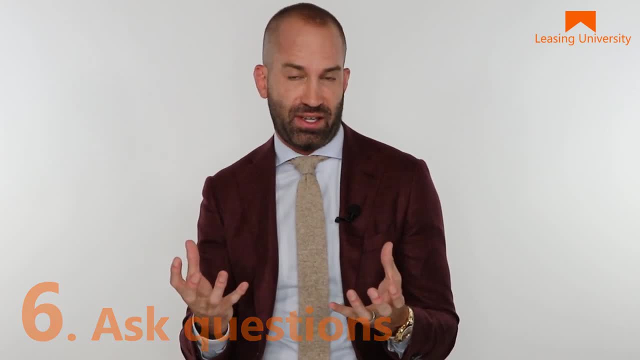 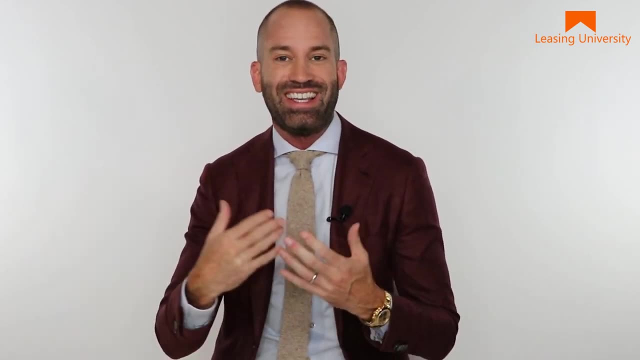 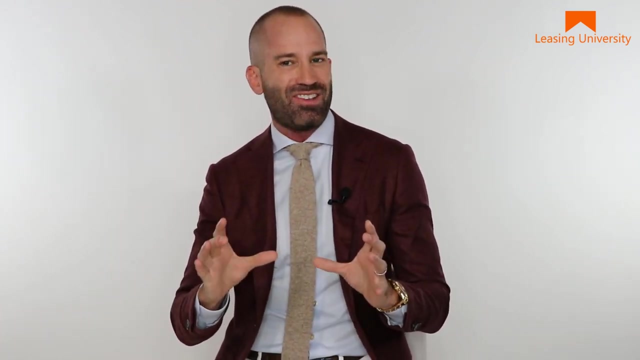 so you're knowing what those power questions are to ask. if you don't believe me that this is an issue, I want you to pretend you're a renter and call some apart. make communities in your market, call any apartment community, for that matter, and you're gonna find that the questions that they ask, well, they're a bare. 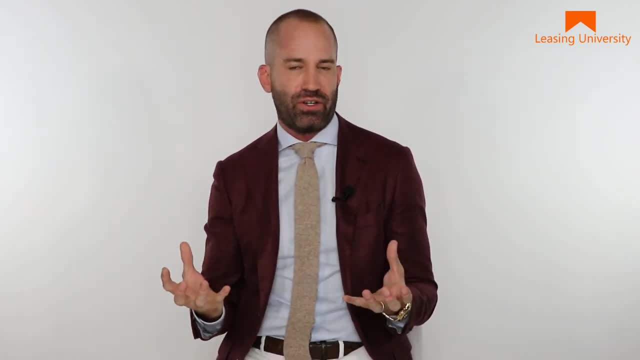 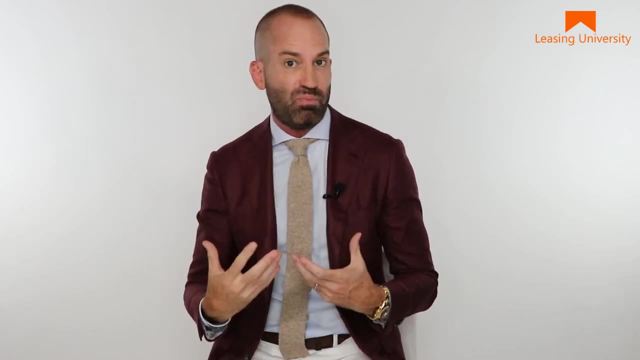 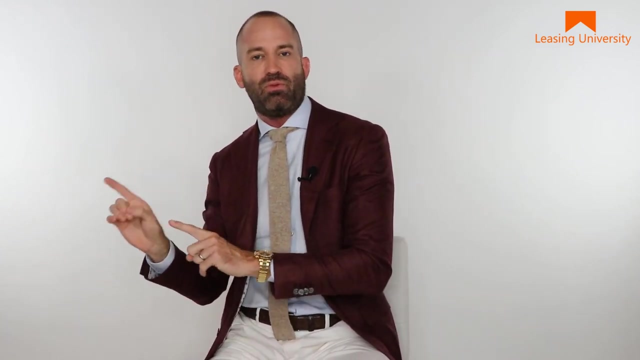 minimum and they're not the right questions to really learn about you. you want to make sure that you have a process that is designed around very specific questions that are gonna help you deeply, deeply understand your prospect, and that's what's gonna help you close the lease later on in the 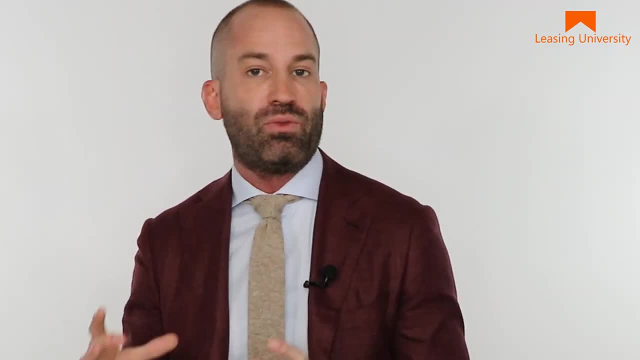 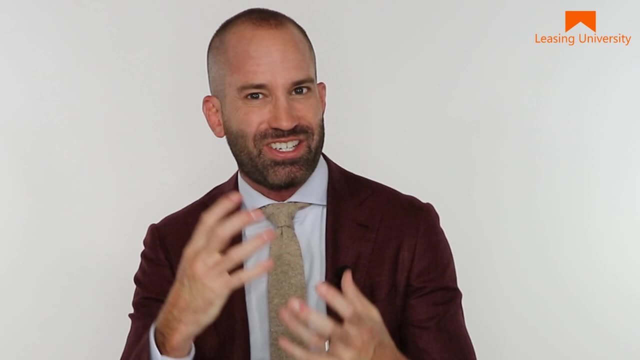 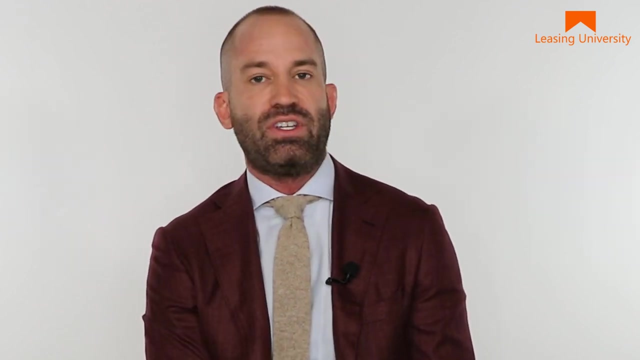 sales process. the data shows that top performing real estate professionals, top performing property managers- well, they're asking a lot more questions, they're digging in there, they're gaining those insights to learn about their prospects. if you're doing most of the talking, you're not a top performer number seven, don't be. 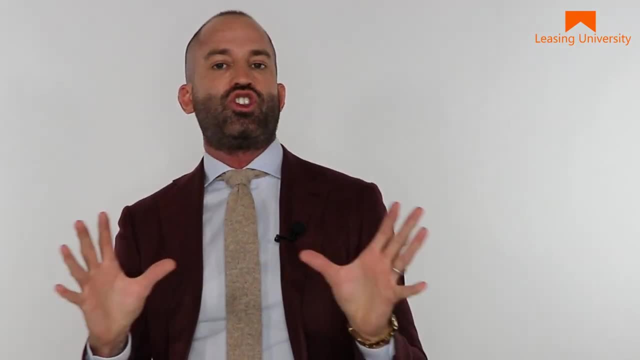 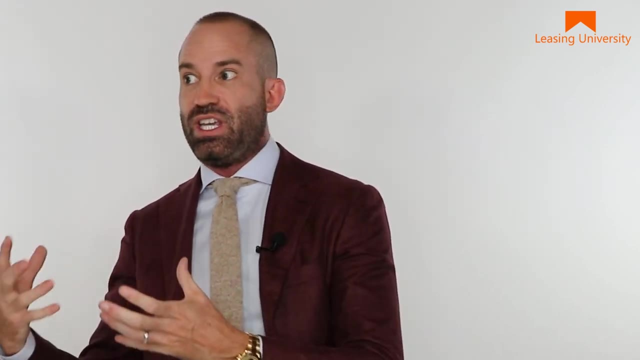 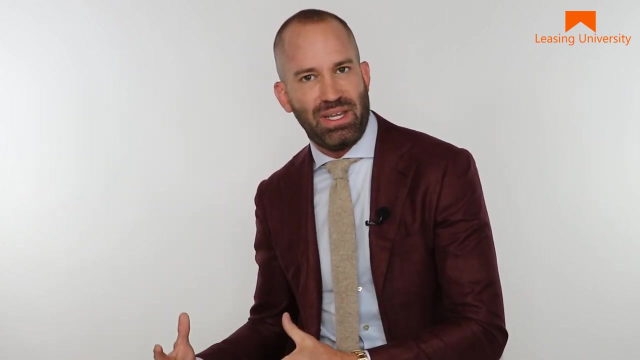 afraid to lose the lease. I find that so many property managers and leasing agents are terrified with the idea of losing a prospect, losing that lead not getting the lease signed. but the fact of the matter is it happens. it's not a big deal. I lose deal sometimes if you have a process that you can trust. if you have a process. 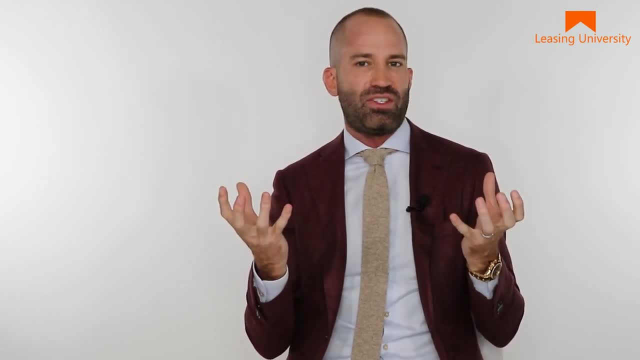 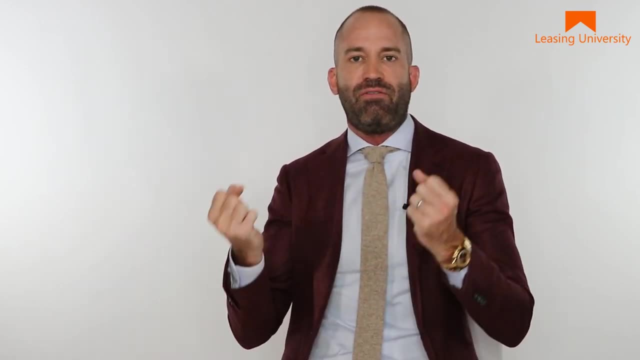 that knows, is gonna figure out whether or not this prospect is the right fit. well, you can go through your life without having fear, without being afraid. fear cripples us as property managers. fear cripples us as leasing professionals. Less Loss多事宜, Less Williams And More火. 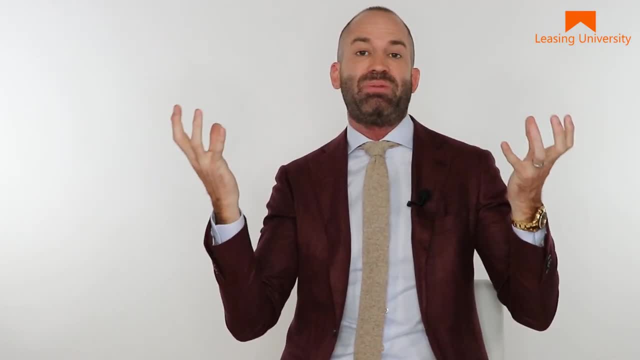 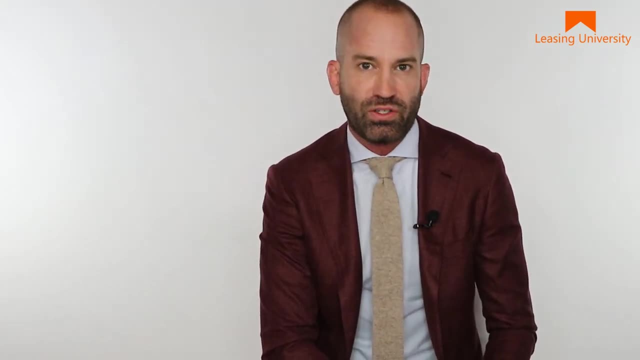 professionals, Our prospects are already in a deep state of fear. If we're afraid that, hey, I'm not going to get this sale, it's only going to make matters worse. Number eight: be a peer, not a servant. When you behave like a peer to your 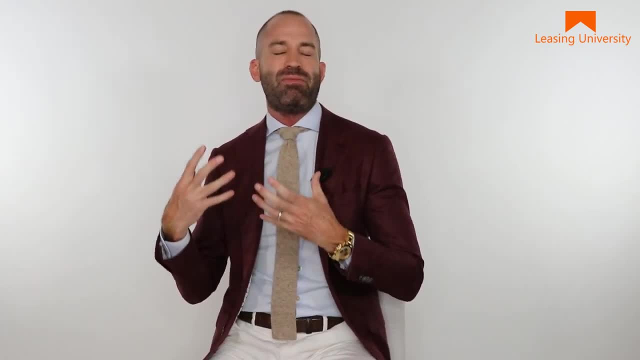 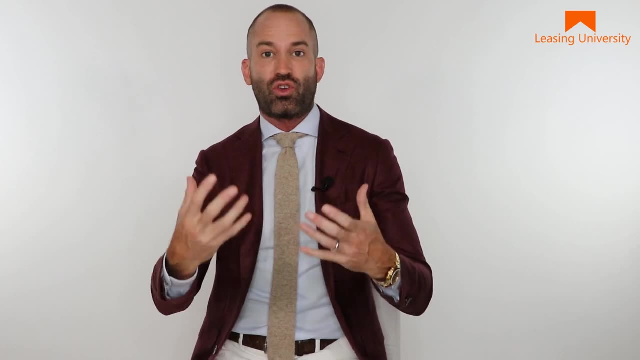 prospects. they feel that and it's disarming and it makes them more comfortable. It makes them feel like, wow, I can really trust this person. They're not just telling me something because they're trying to tell me what I want to hear. They're telling me something because it's the truth. Make sure that. 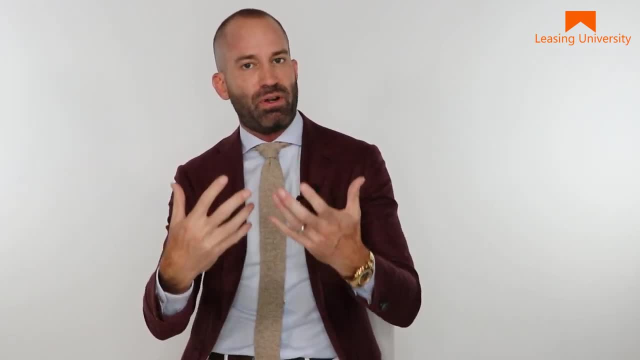 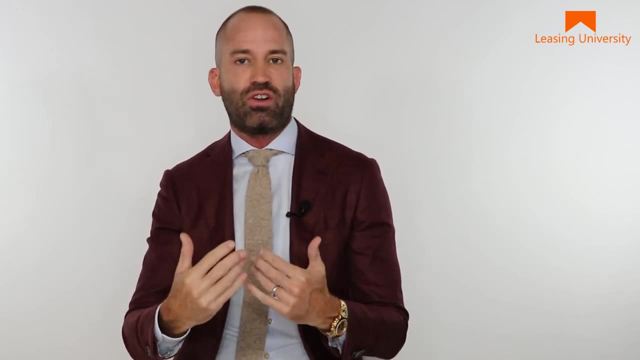 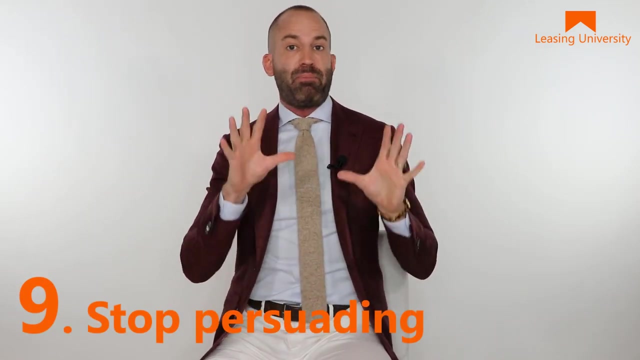 you're treating your prospects as an equal. You're a professional and they're your client, and you're working with them as a peer, versus you're just a servant that's there to get them exactly what they need and tell them the answers that they want to hear. Number nine: stop persuading Your prospects. don't need to. 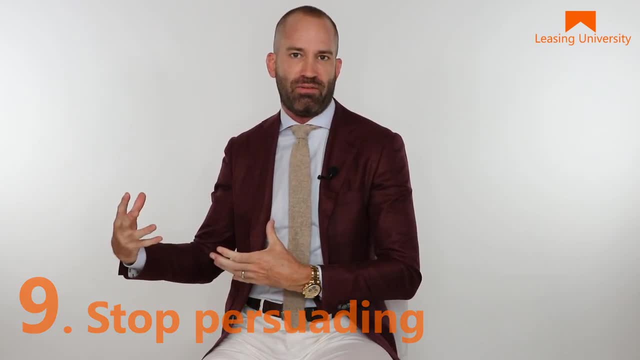 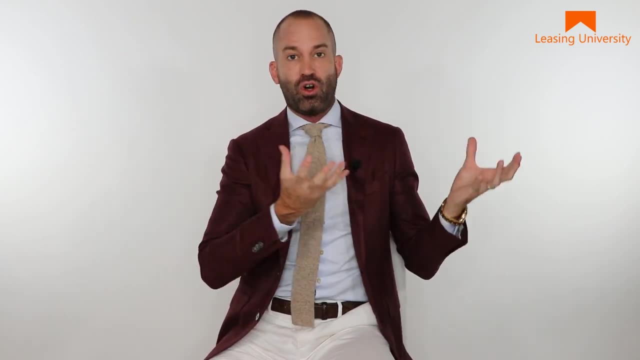 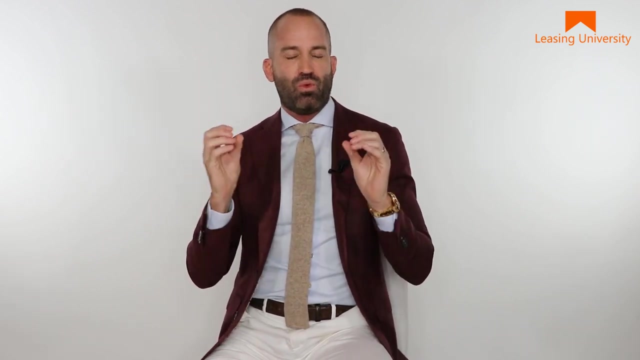 be persuaded into renting an apartment from you. What they need is an answer is they need that trusted advisor that's gonna really look at their situation, look at all the alternatives and help them decide on the best possible outcome for them. Think about this. 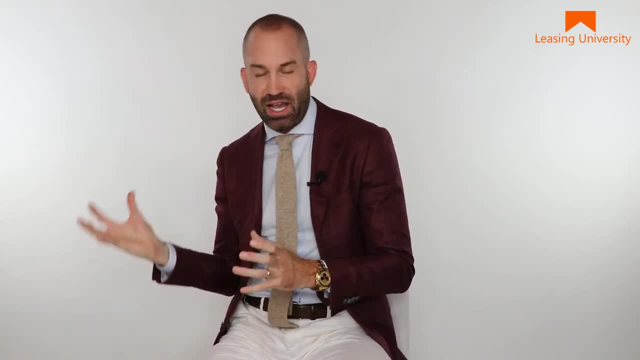 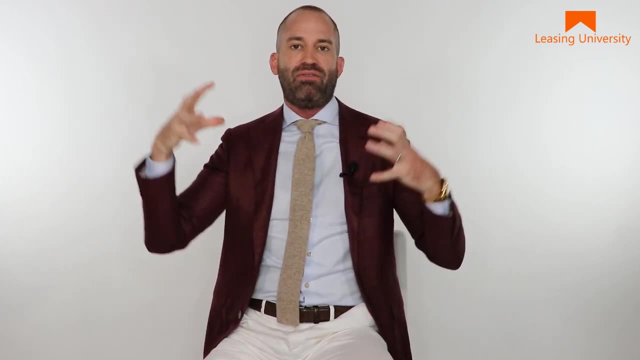 They're gonna have to go to bed in that apartment every single night. They're gonna have to wake up there every morning. They're gonna build their life there. It's literally going to be the center, the focal point of their entire life. 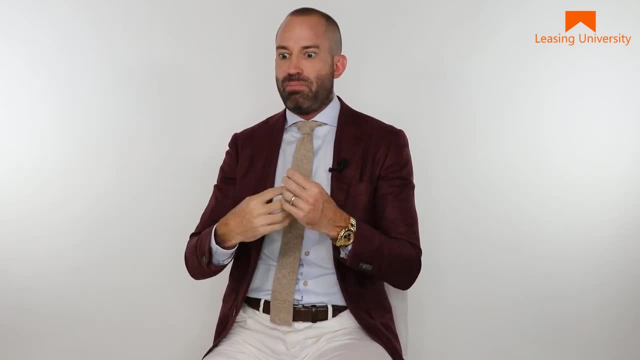 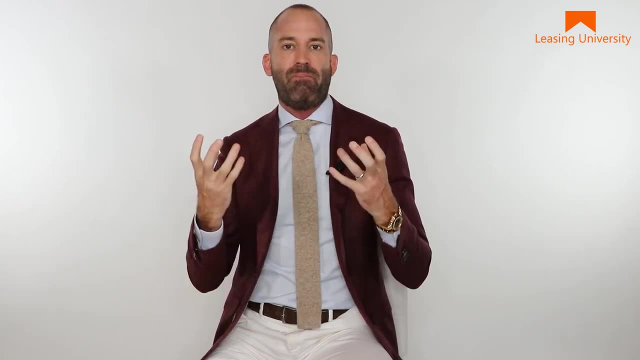 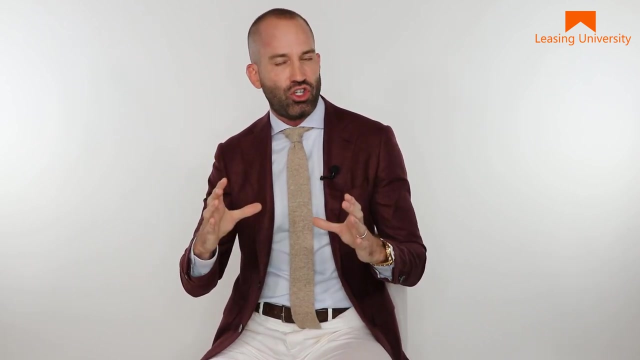 They don't wanna be sold or persuaded or be given some tricks or gimmicks to rent the apartment. They wanna make a good, sound decision, based on facts, based on data, based on your understanding of their situation. So make sure that you have a closing system. 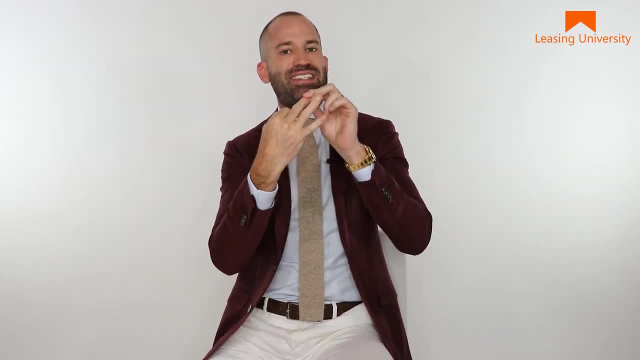 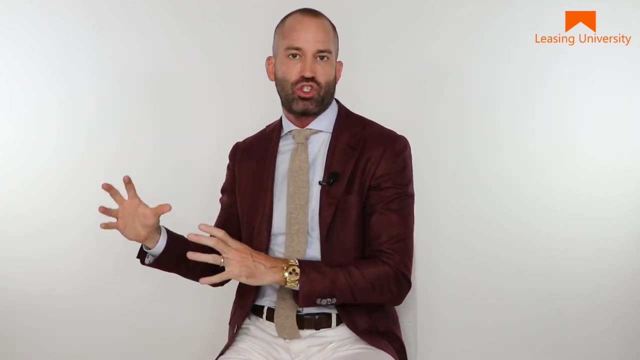 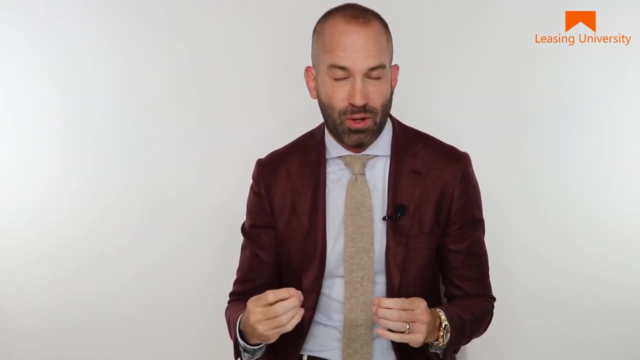 that's not high pressure, it's not manipulative, it's not pushy. okay, If you're not gonna use our closing system, go find one that is not based on persuasion Your prospects. don't wanna be persuaded, tricked, pushed or manipulated into renting the apartment. 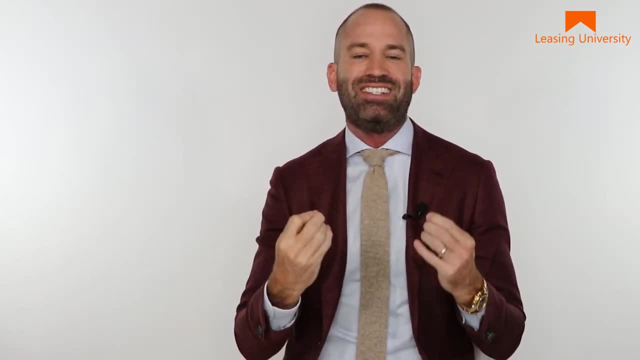 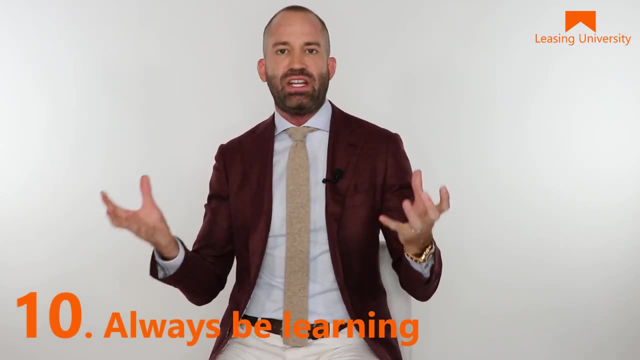 They wanna make that decision on their terms, because it's the right decision to make. Number 10, always be learning. Learning is a lifelong journey and our industry is constantly changing. You can always get better, You can always improve If you have that attitude. that 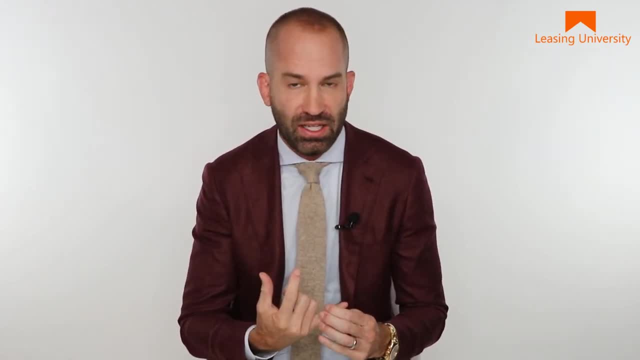 hey, you know what? I learned a little bit when I first got involved in the industry back in 1992.. I learned a little bit when I first got involved in the industry back in 1992.. I learned a little bit when I first got involved in the industry back in 1992.. 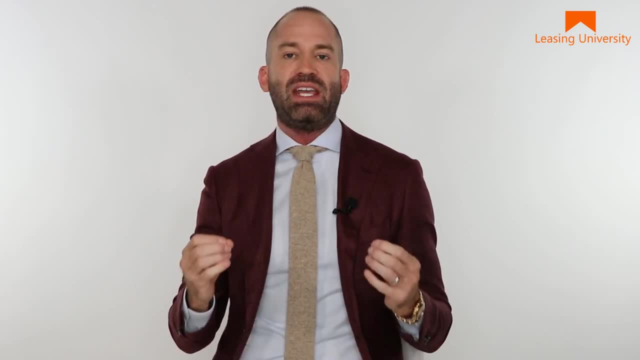 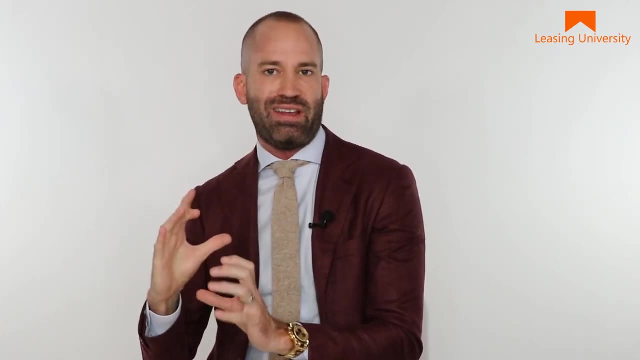 And I know everything. Nobody knows everything. Make sure that you're spending time each and every day to just learn a little bit right? If you can just get 1% better every day, your career is going to go through the roof. 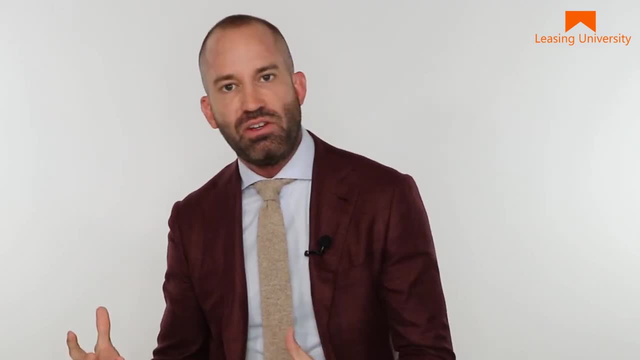 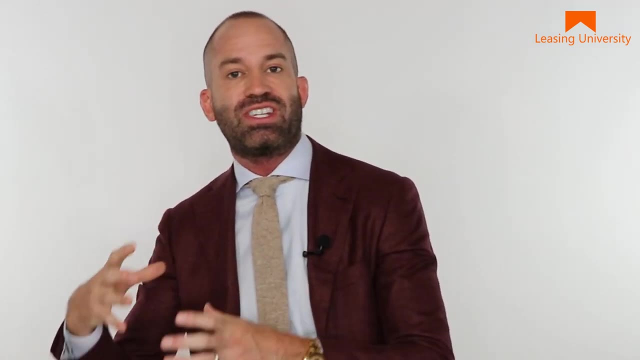 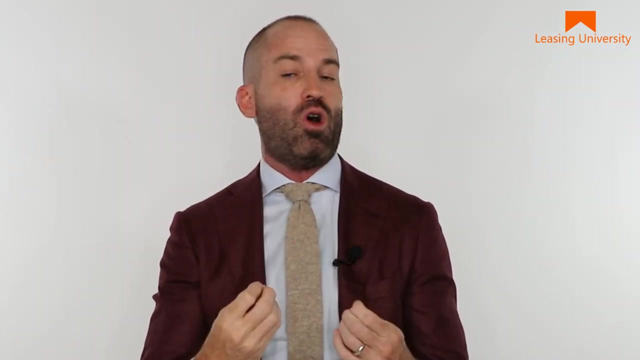 Find like-minded people that are excited within your company to learn new things, to try new strategies, to improve their process. Be around those people, Stay positive and always be learning. Trust me, you're going to make so much more money. You're going to have so much more fun. 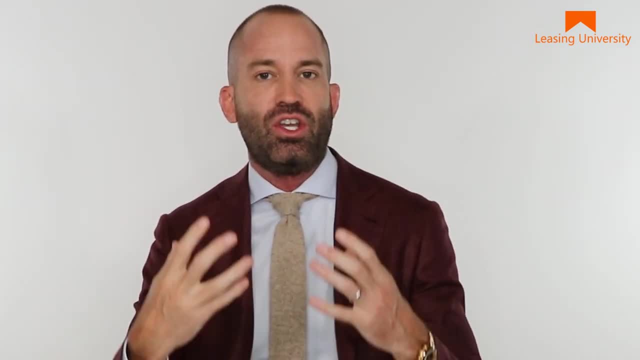 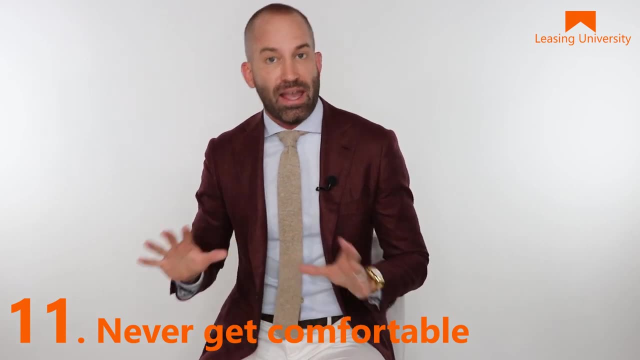 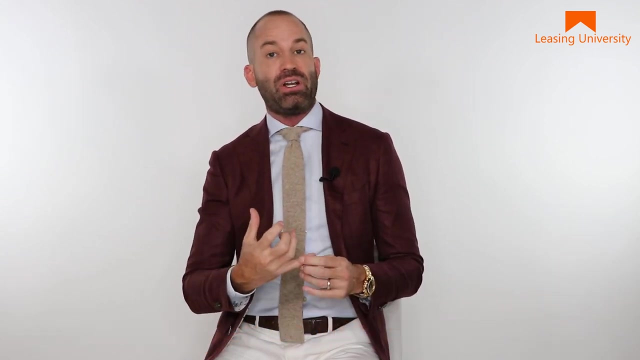 if you're constantly open to new ideas, new strategies and new techniques. Number 11,: never get comfortable, ever, Because when you get comfortable, that's when you get into trouble. I see this all the time, right? Property managers, leasing agents. 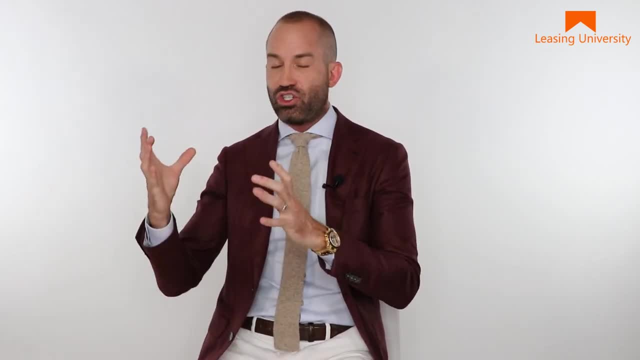 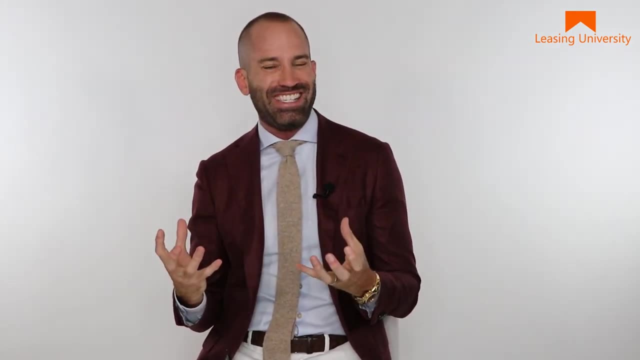 maybe you're in a really hot market right now. Maybe you're in charge of a lease up. that is the place that everybody wants to live at- And those leases are coming a little bit easy, right. You start to get comfortable, You start to get a little bit lax. 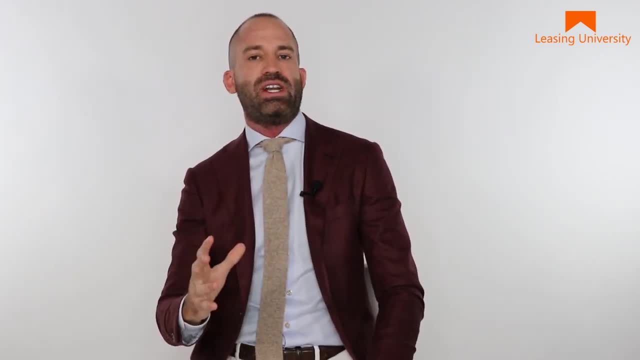 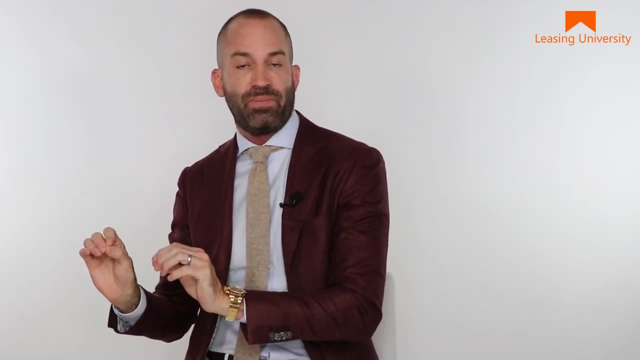 You maybe don't run to grab the phone because you're not worried about your property getting to 98,, 99, or even 100% occupancy. As soon as you get comfortable, things are going to start to decline, And this is so important for you to realize. 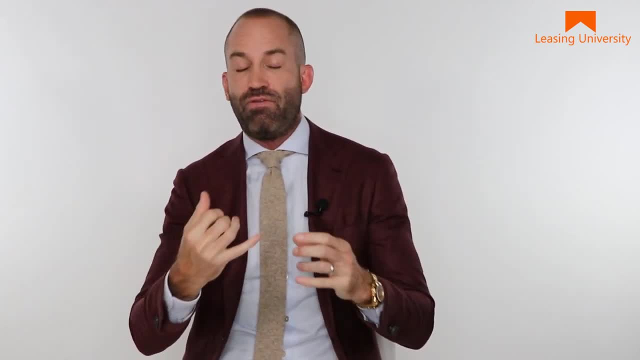 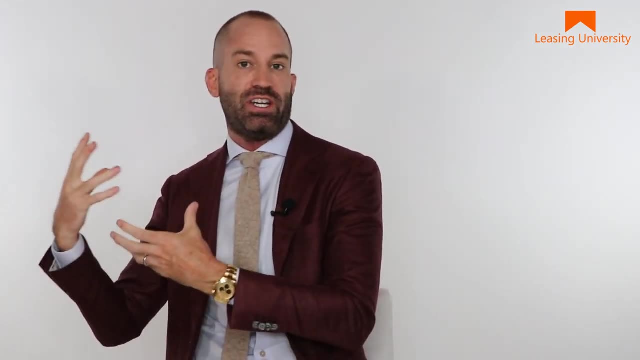 Because if you find the right sales training system right, You find a system that's going to help you. You find a system that's easy to learn, easy to implement. You find a way to close these prospects that's not pushy, not manipulative. 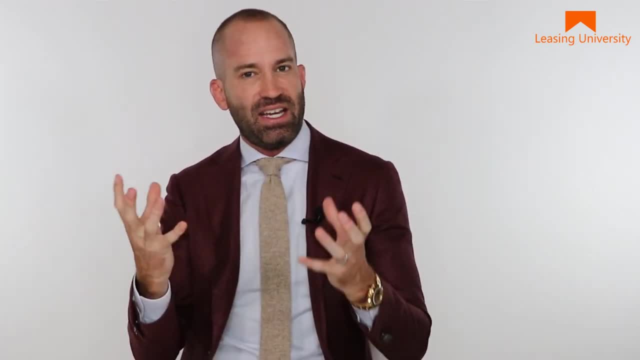 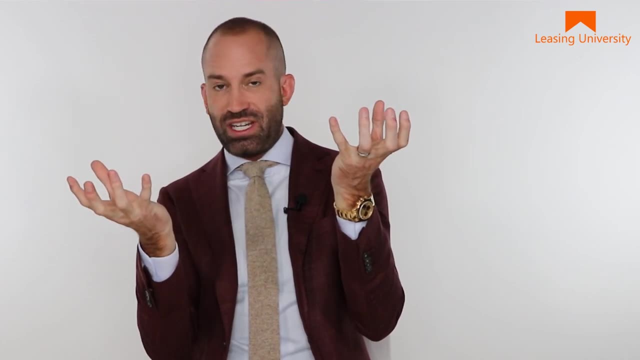 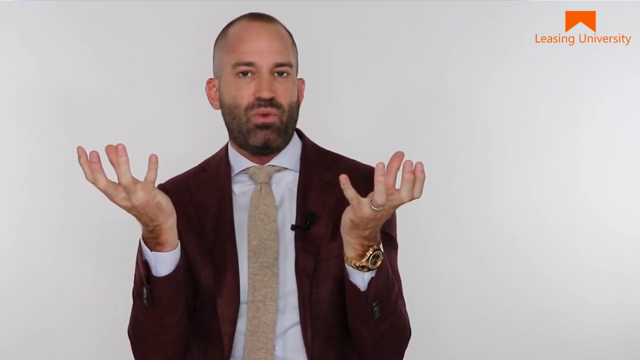 Well, guess what? Your job is going to start to get easy, And it's this weird thing that happens: as your job starts to get really, really easy, You actually start to get comfortable and you start to do less of the things that made your job so easy to begin with. 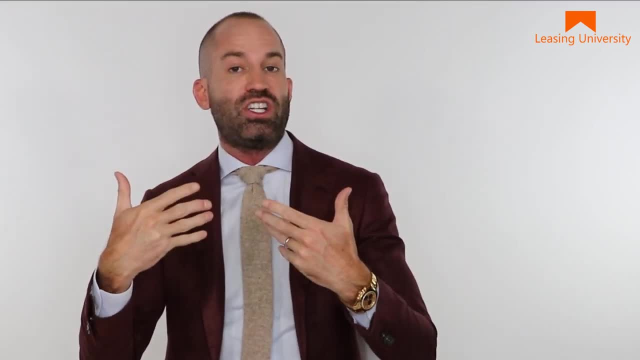 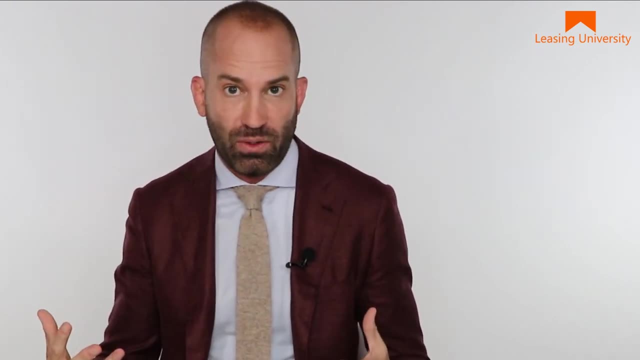 Find that process And when that process starts to decline, it starts to give you results. Don't get comfortable, keep it up. It's like people that get on a diet and they start to lose a little bit of weight, right, Or they start to build a little muscle.